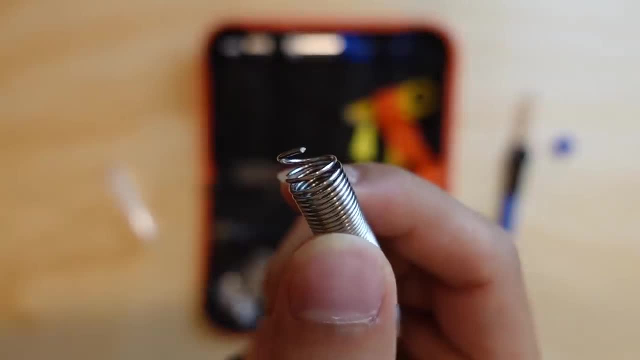 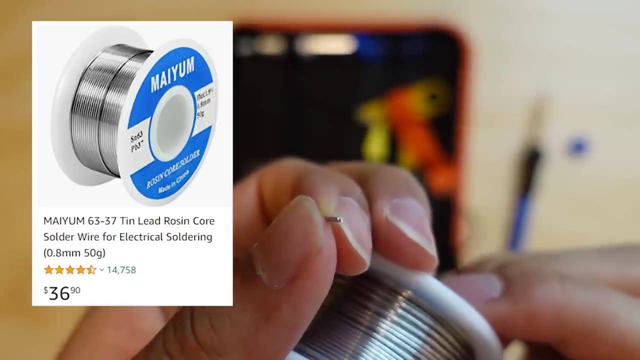 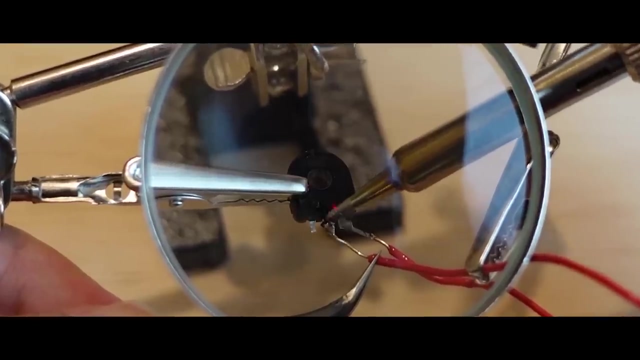 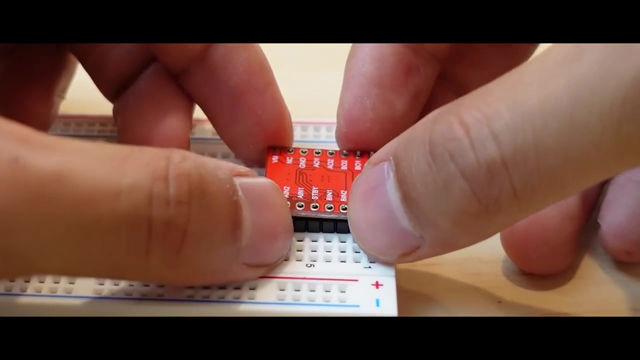 the cheap included solder that comes with the kit doesn't have the flux, And to buy one that does it only costs like twice the amount as the whole kit. Hey, capitalism. Anyways, here's the soldering. Let's play it. I shot through the sky. I'm stuck on the ground. Why do I try? I know I'm gonna fall down. 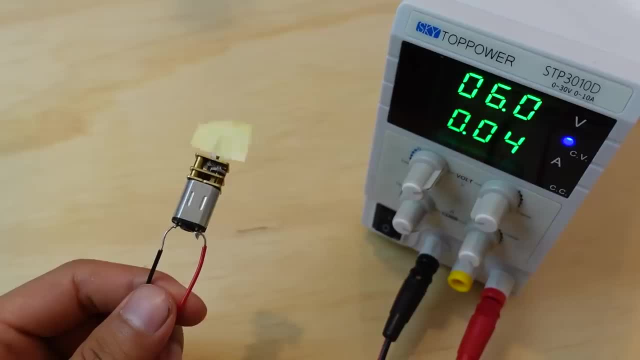 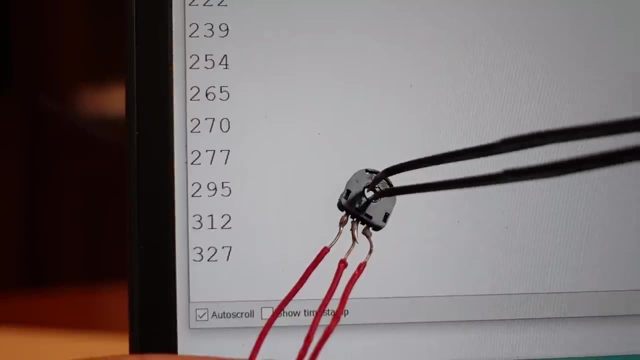 Let's play it, Let's play it, Let's play it. that that's done. we can see that the motor spins, the motor driver controls the direction which it spins and the potentiometer helps read what angle it's at. my iq is approximately 3000, so i combine. 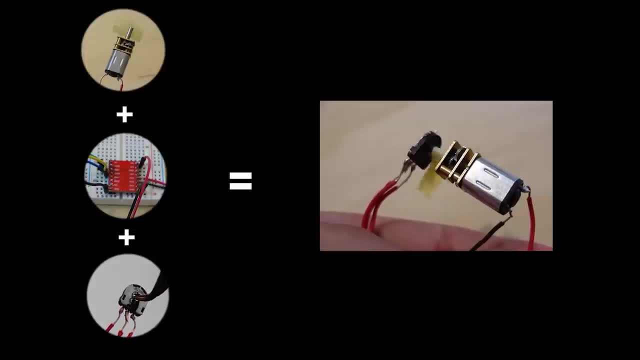 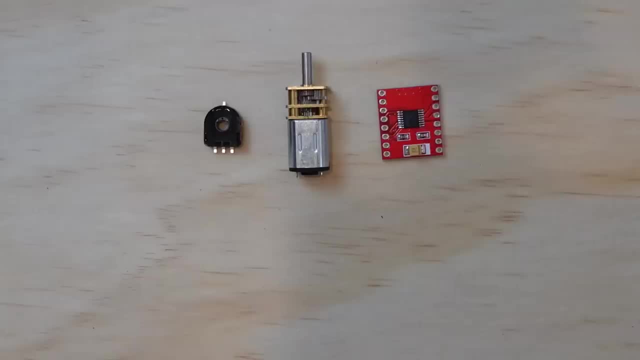 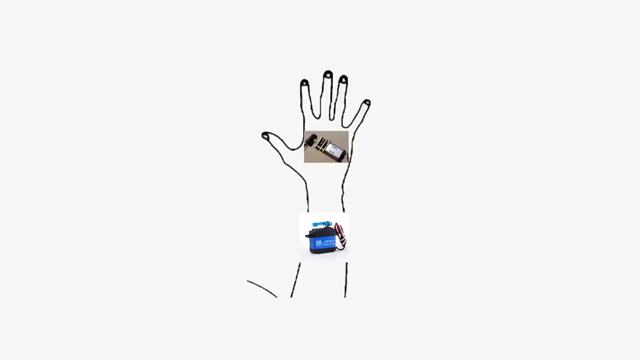 the functionality of all these parts to be able to control the angle of the motor shaft- basically recreating a servo. okay, so why don't i just use a servo? well, look at this, the servo is way too big. these smaller parts are able to fit into the palm of the hand instead of having to go in the forearm. 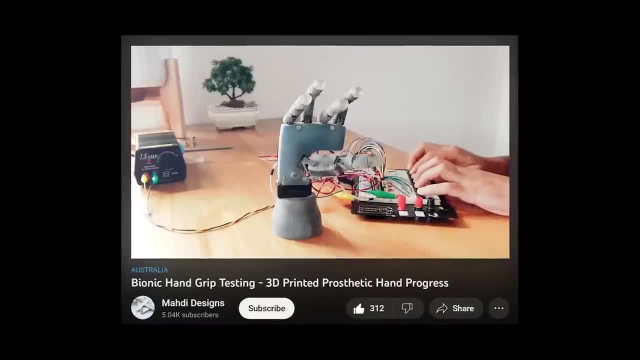 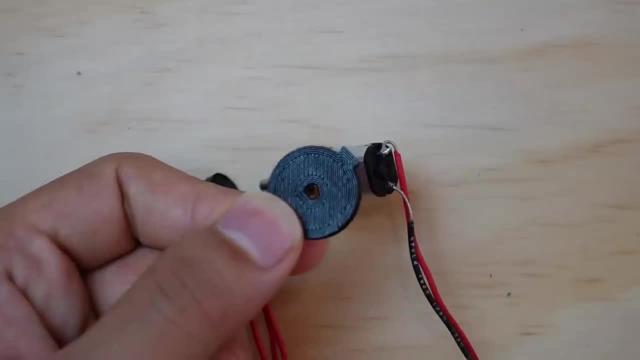 so the final product can be a lot more compact. credit where credit is due. this great design idea came from madi designs, who's also making a bionic hand link in description. so i made this little pulley wheel thing to help pull the fishing line. but one issue i ran into was that the d shaft 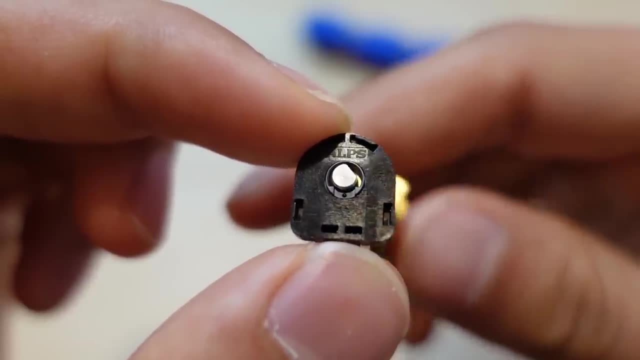 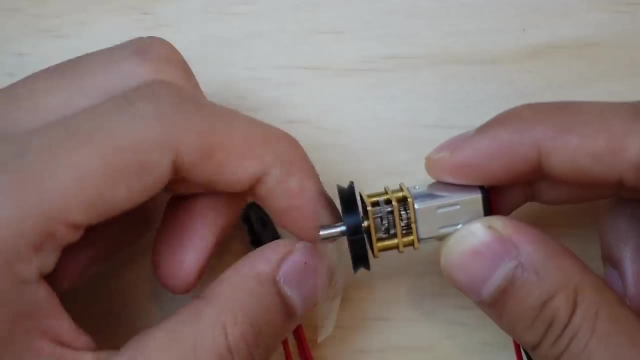 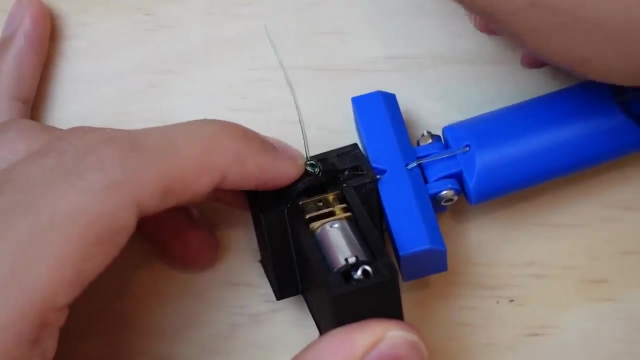 of the motor was not actually big enough to fit into the angle sensor, so it wouldn't rotate with it damn. but surprisingly this was pretty easily fixed with some tape. now i just had to thread the line through and tie a knot to secure it, and then the parts fit into this little box. upon testing, the 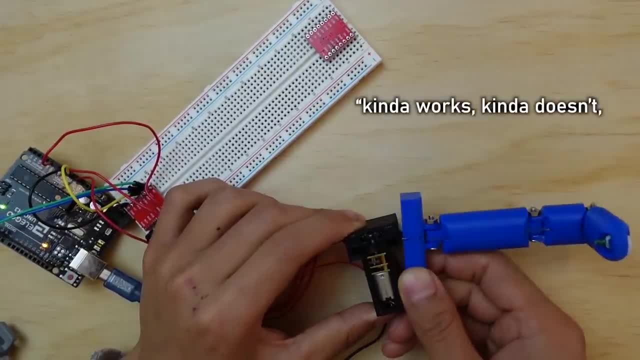 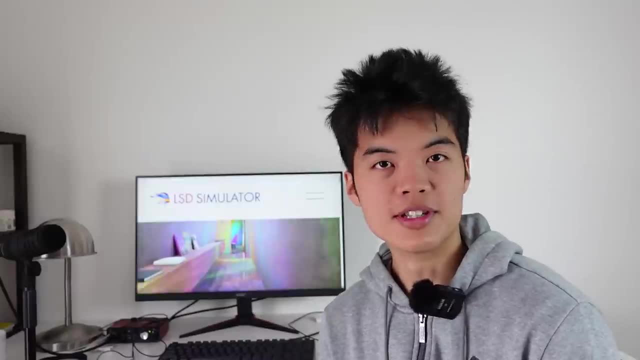 contraption was once again in the state of kinda works, kinda doesn't. but don't worry, we'll fix it later. in other words, it's perfect. my friends, here is where everything goes south. you might notice that my hair is a bit longer, and that's because 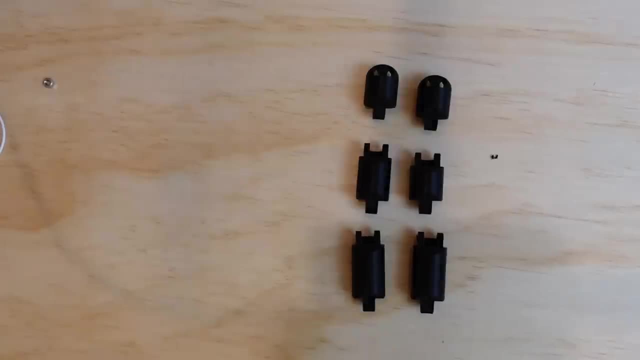 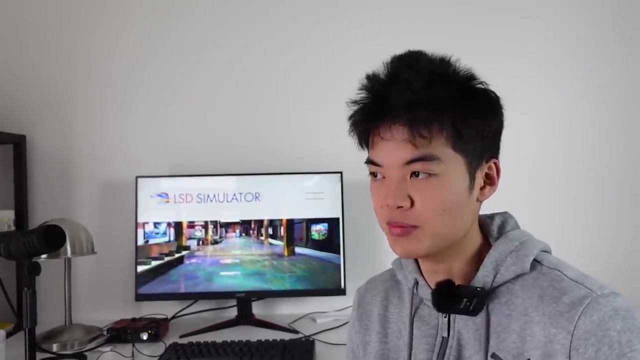 it's literally been weeks since i filmed the last bit. so what happened? well, first i made more fingers, plus a palm component to fit all the motors in which, by the way, do you know how hard that is for someone like me who dropped out of school, to do crypto? it's not like i'm any good at 3d design, so 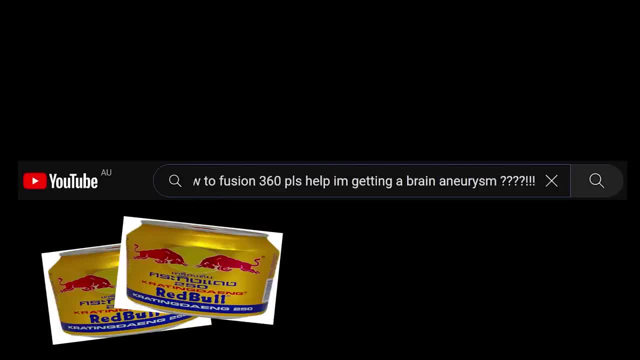 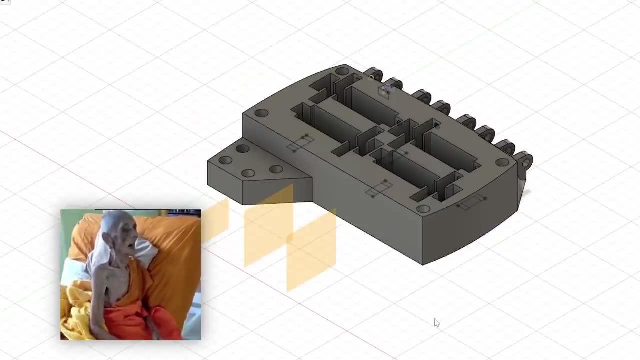 i needed like 69 youtube tutorials and two packs of red bull in the process. when i first started designing it, this baby looked like this, but when i finished, it looked like this. this is luang pho yai, a buddhist monk. anyways, that's not even the main problem, probably not. the main problem is that 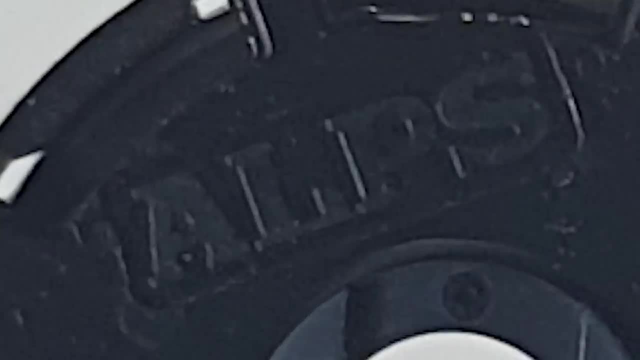 it's not even the main problem. is that it's not even the main problem? is that it's not even the main problem? the guys at alps were probably smoking weed when they designed this potentiometer, because who the puts a cutout on the side that's supposed to be flat? that was causing problems. 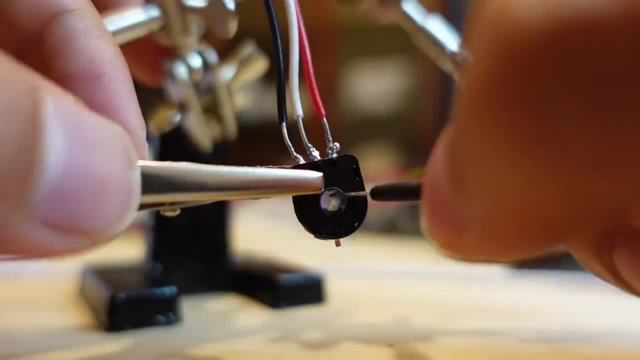 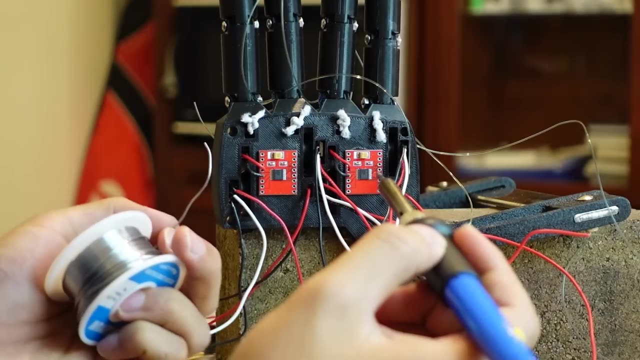 even with the tape. so i had to try all sorts of goofy ways to fill it up and in the process accidentally jammed four of them with the epoxy resin. rest in peace. problem number two: i tried putting the motor drivers on the hand itself to save space and to look cool for the thumbnail. 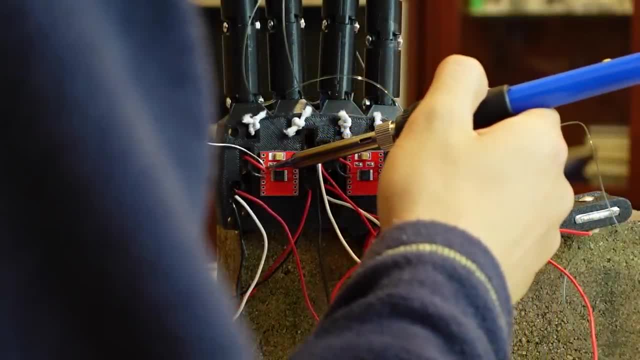 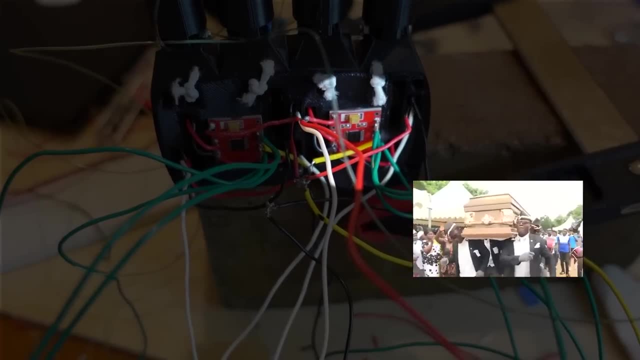 but that just over complicated it because i had to do so much soldering in such a small space and i think i accidentally broke one of the motor drivers because it just stopped working. i don't know, maybe i overheated it with the soldering iron or something. but let's be honest, when the wires 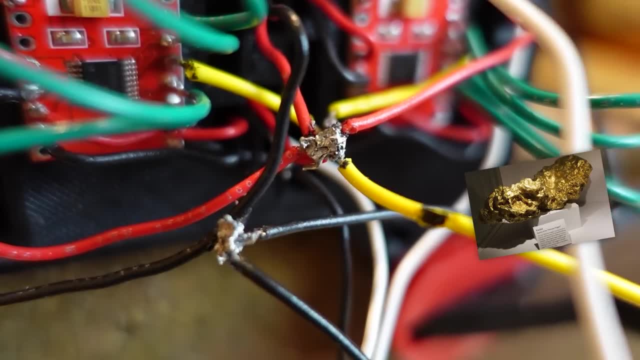 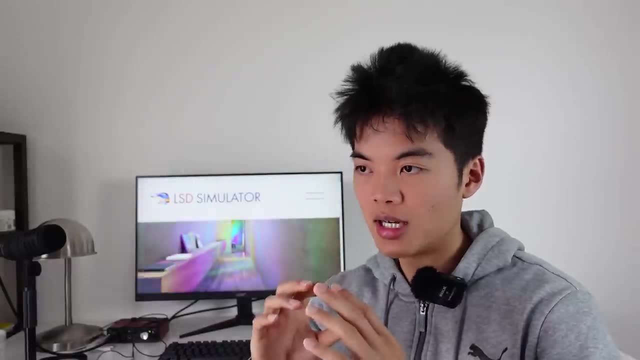 look like expired spaghetti bolognese and the soldering looks like prehistoric metal nuggets from the asteroid that killed the dinosaurs. you know it's about to fall apart at any moment. okay, so let's break this down logically. i tried putting the motor drivers on the hand and that was too much. 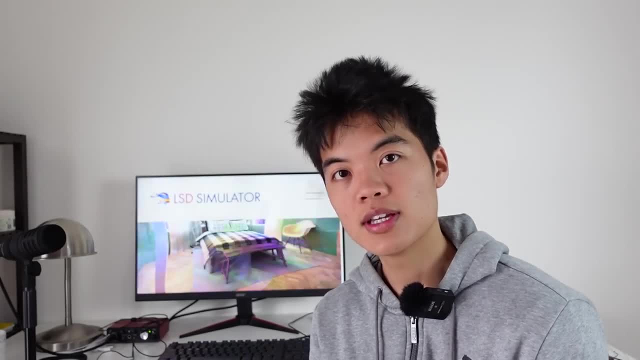 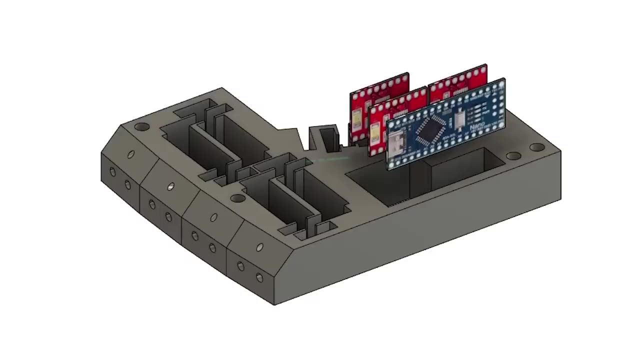 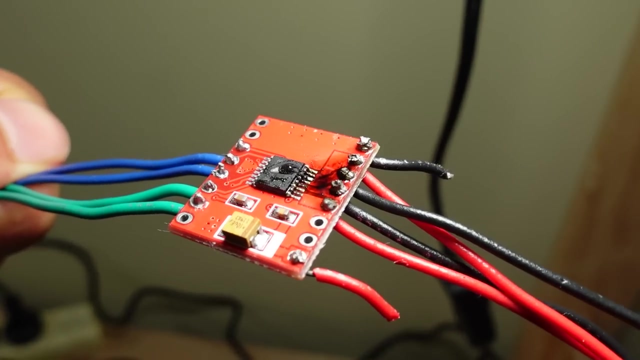 in too small of a space, which resulted in the whole thing failing. so i used my problem solving and i connected the dots for this one and had a good think about it, and i thought i'll put the arduino in there too. it'll look even cooler. why are we still here just to suffer? yeah, so now i 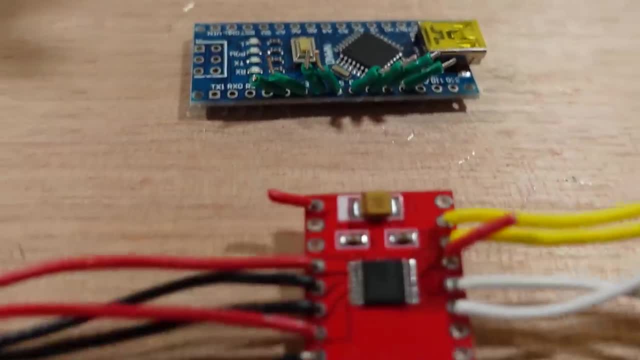 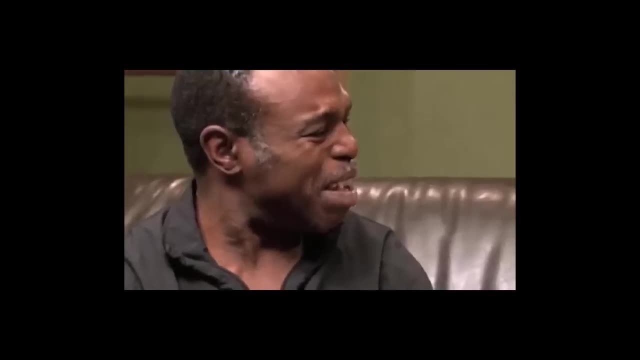 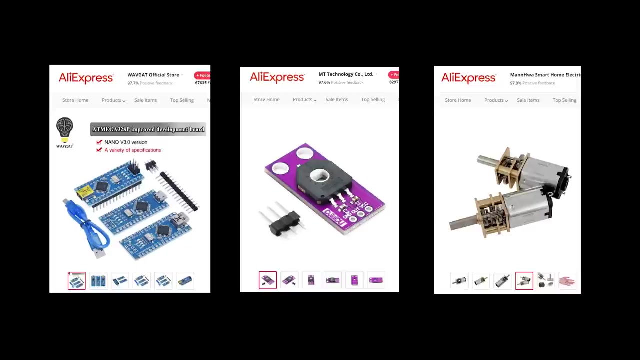 blew up. one motor driver from a short circuit got a bunch of wires stuck on these components which i can't be bothered to remove, and overall wasted enough wires to rebuild a sci-fi version of the roman empire. i decided to restart. i ordered some new parts from aliexpress, but they were going to 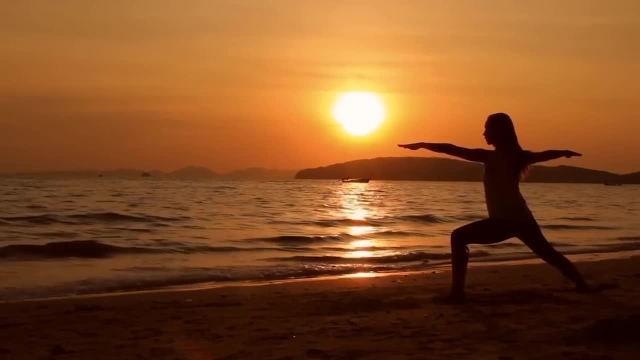 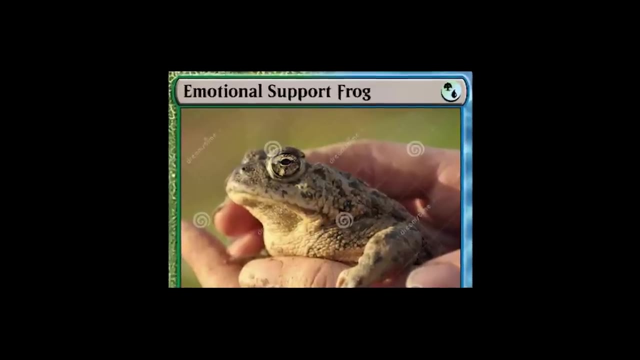 fail. so in the meantime, it was an opportunity to take a break from all this difficult engineering, recover from burnout and regrow some brain cells in need of a bit of emotional support. i turned to the chat gpt ai because, well, let's be honest, it's not like i have any friends in real life. 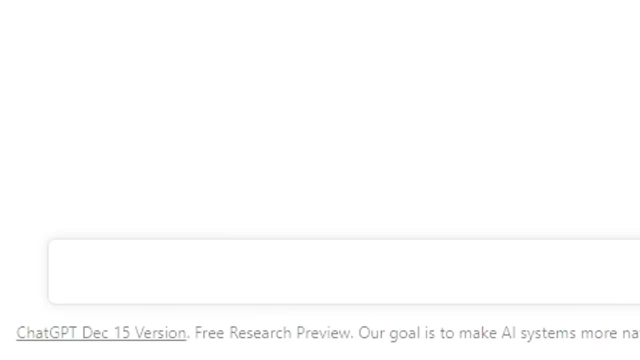 let's start off with the main question at hand: why am i so ass at building robots? it's not uncommon for people to feel like they are not skilled at building robots, especially if they are just building robots can be a challenge. oh damn, it's actually giving some good advice. well now how? 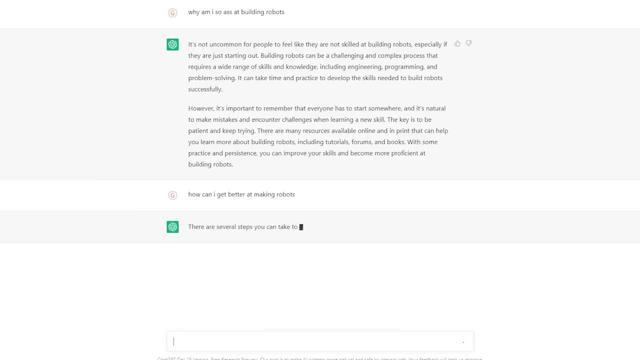 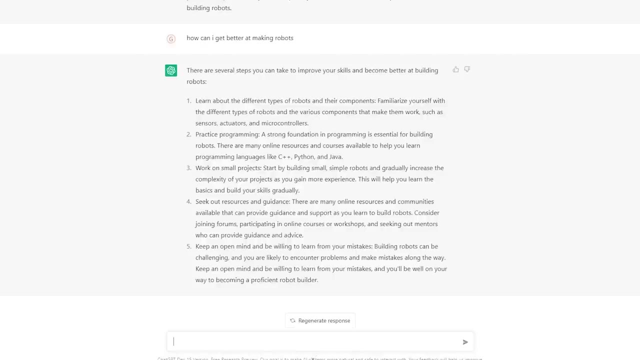 about: uh, how can i get better at making robots? there are several steps you can take to improve your skills and become better. oh wow, i was just gonna use this as a skit for the video, but it seems like it actually has some good answers. i should probably ask some like actually important. 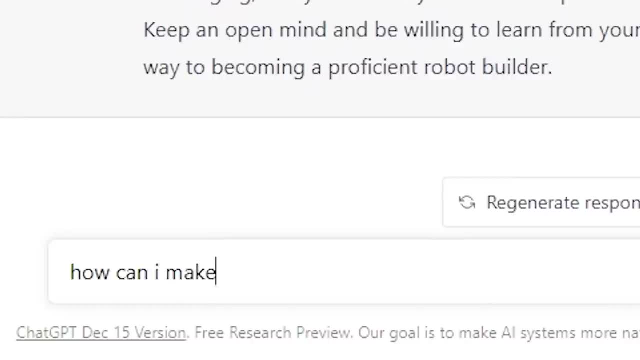 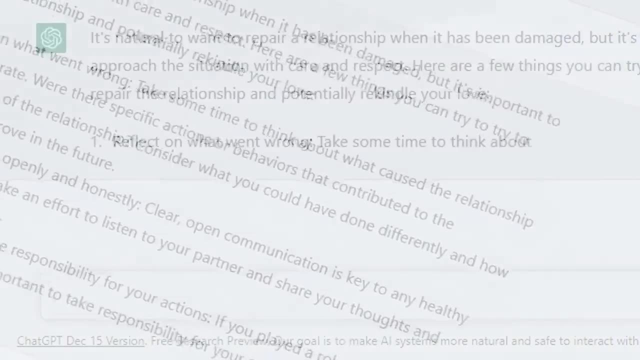 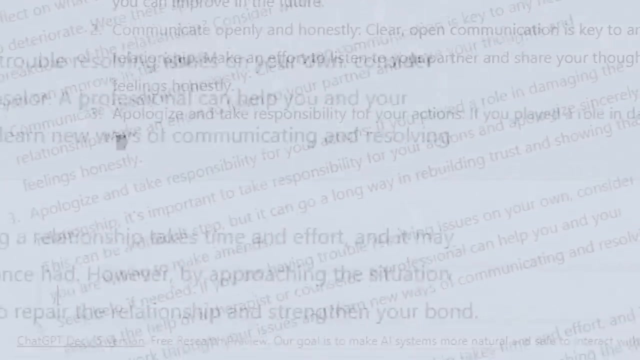 questions it might be able to help me. it's natural to want to repair a relationship. when it has been, you can try to try to repair the relationship and potentially rekindle your love. open communication is key to any healthy relationship. responsibility for your actions- how you can improve in the. 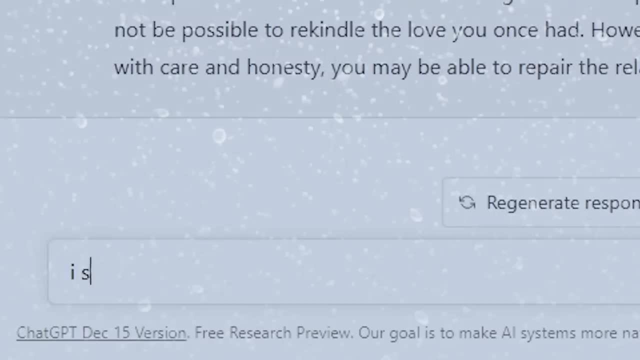 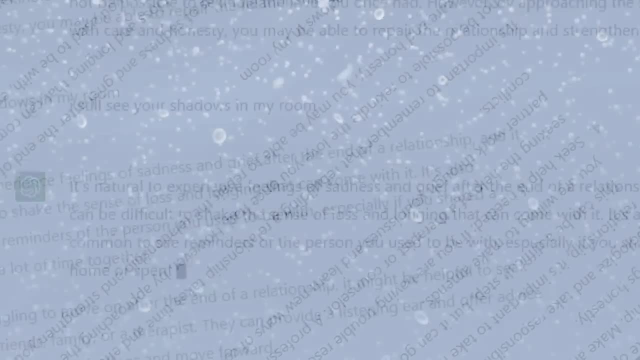 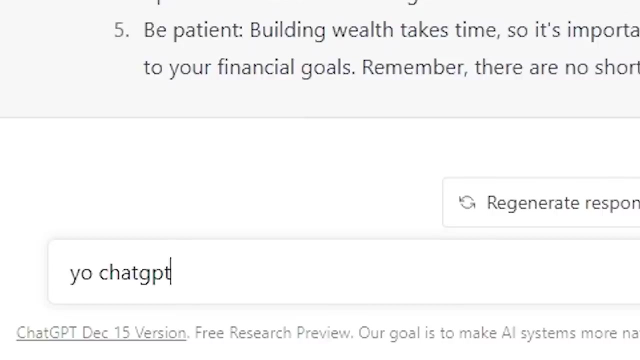 showing that it may not be possible to rekindle the love you once had. it's natural to experience feelings of sadness, reminders of the person you used to be with after the end of a relationship, such as spending time expressing your emotions all right. now watch this. 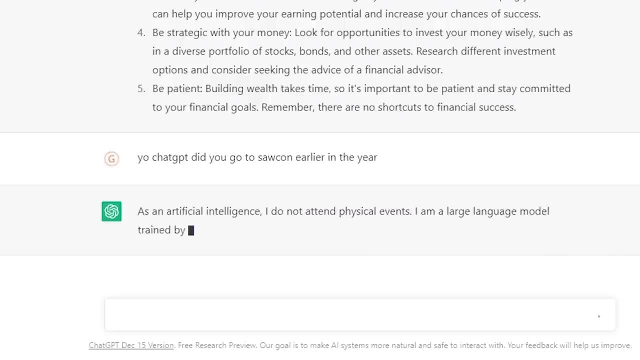 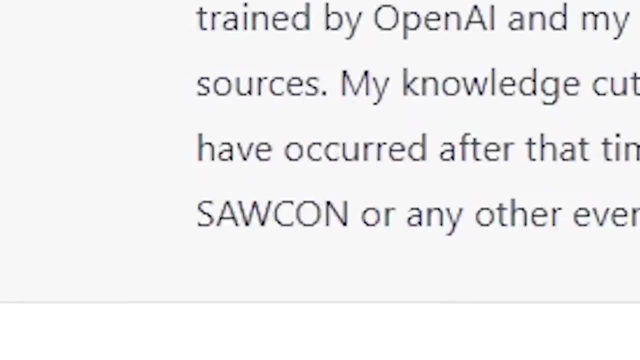 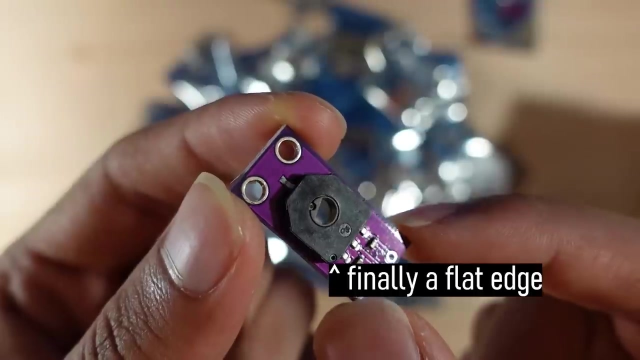 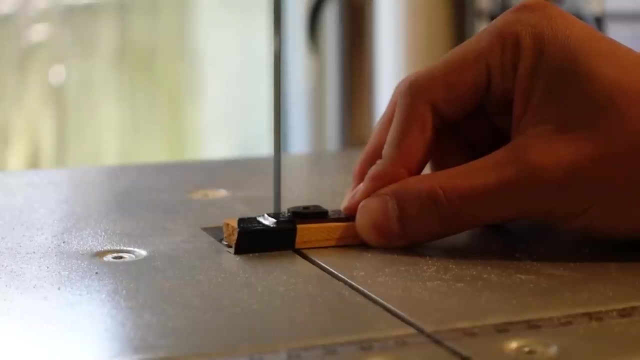 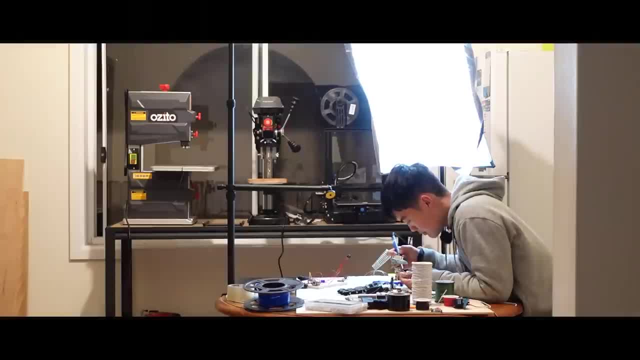 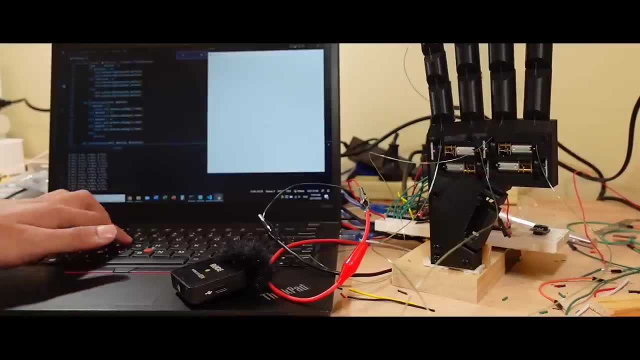 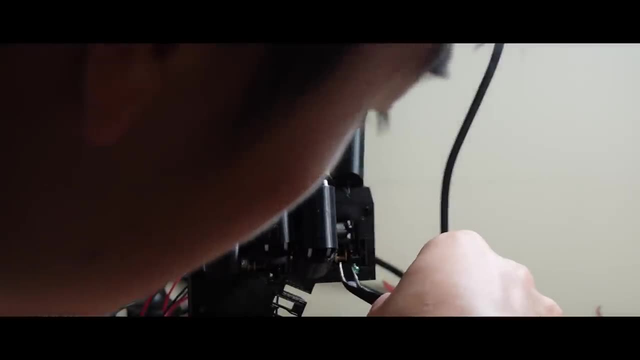 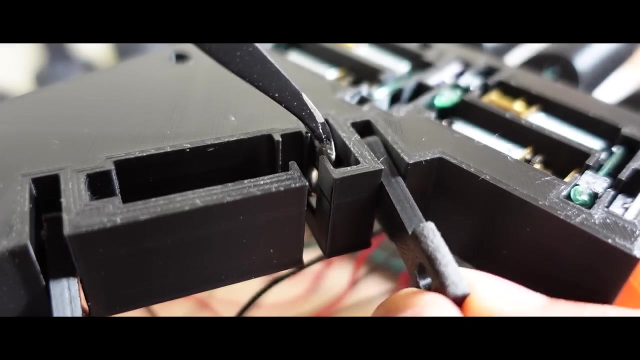 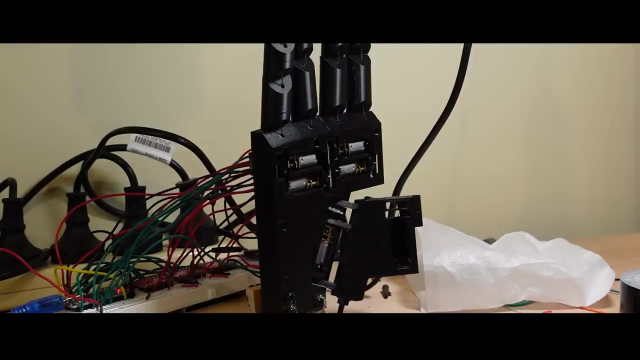 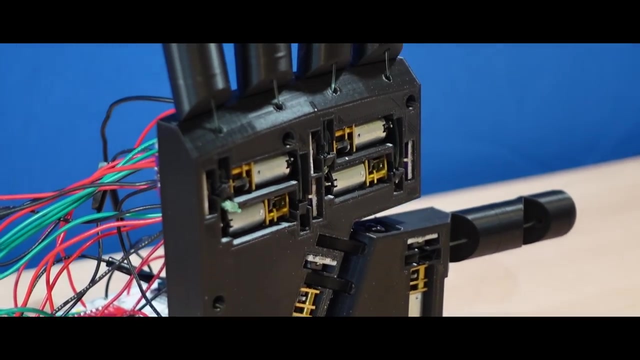 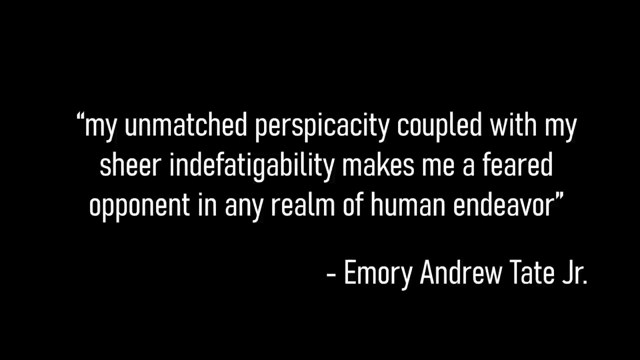 grind again, roll the montage. so so, so. so, ethan, finally, with great effort and sacrifice, we arrive at the finished hand, for my unmatched perspicacity, coupled with my sheer in the fatigability, makes me a feared opponent in any realm of human endeavor, although i guess there's a reason. people design custom pcbs, huh. 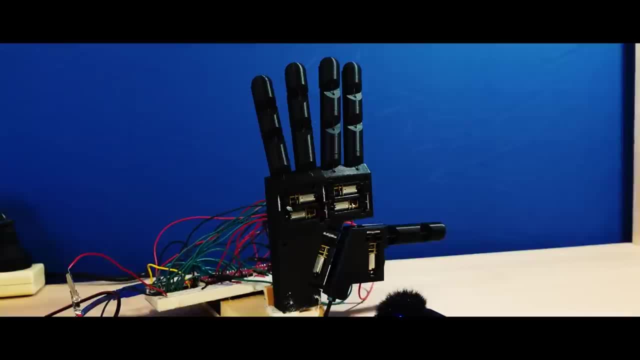 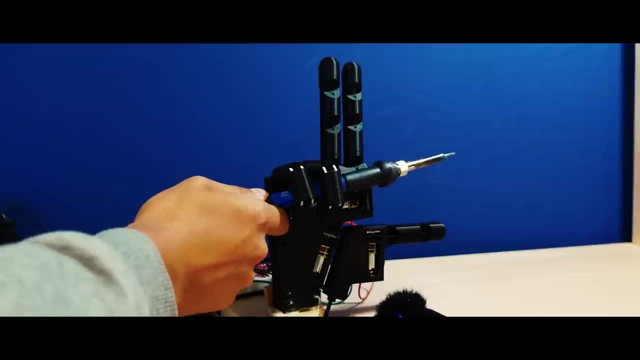 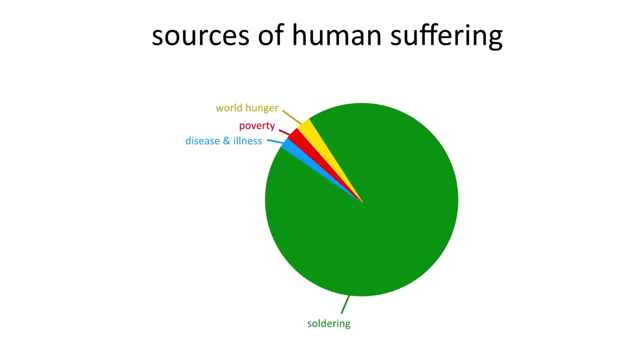 we're back to the breadboard and it looks ugly as hell. anyways, to test out the finished project, i place upon its palm the source of all that suffering through this whole engineering process: the 14 soldering iron i got from ebay, because, oh lord, was there a lot of soldering, i'm convinced. 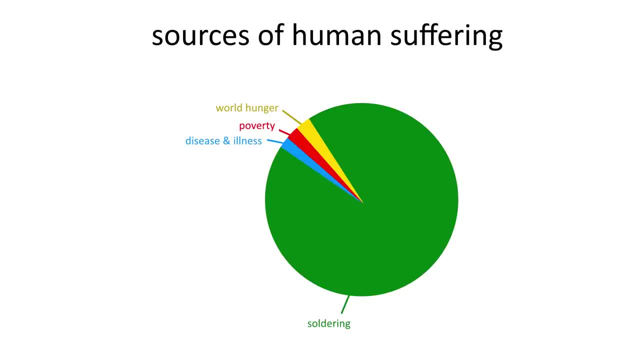 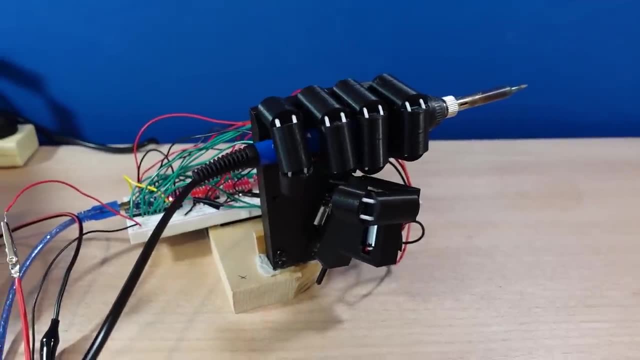 that soldering is the root of like 80 of human suffering. the thumb doesn't even close onto the other fingers properly, god damn. okay, now, after that i need to film the intro sequence. let me give a bit more of a technical explanation now. i managed to write a python program that directly. 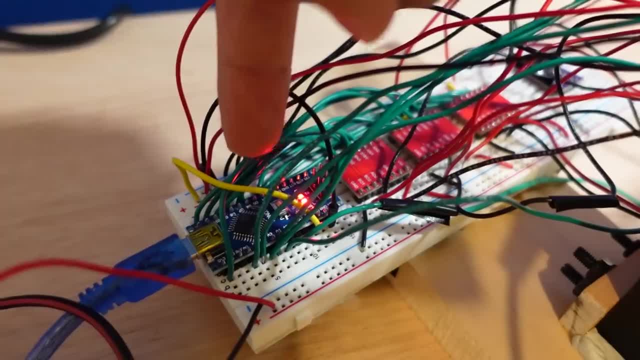 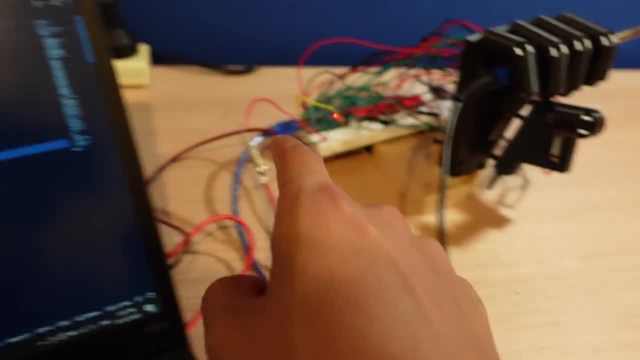 controls the arduino from this computer right here. usually the code has to be run on the arduino, but i found a library called pi from mata, which means you don't have to run the code on the arduino, you can just run it in python. what that means is i can press these keys and that'll. 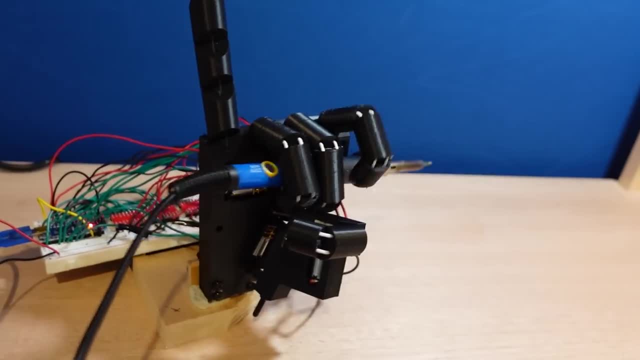 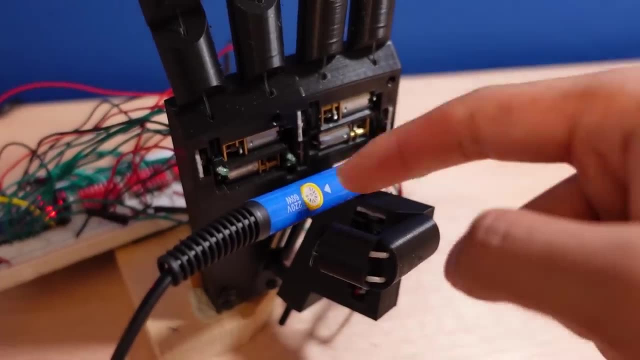 control the motors if i press all of them at the same time. these numbers on the screen are the angle readings from the potentiometers, which play the important role of limiting the angle of the motor so that it doesn't jam its fingers into itself and self-destruct. 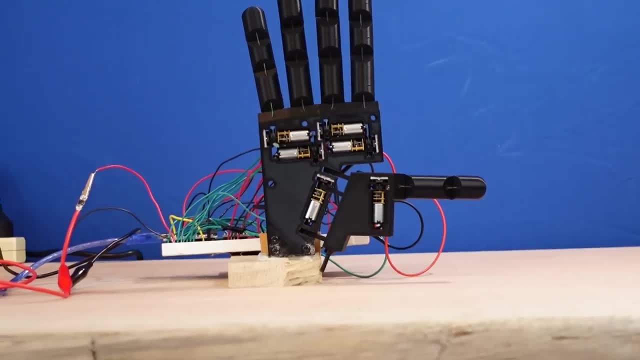 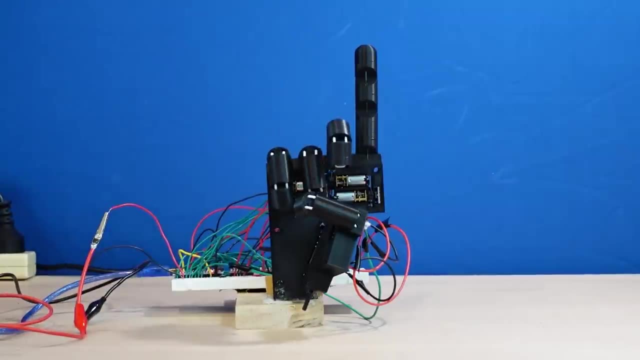 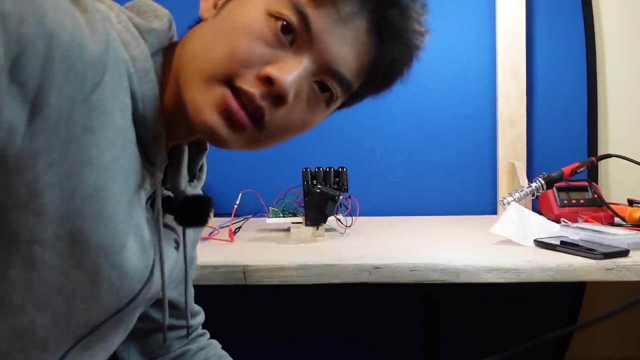 all right. so for the intro we just pan up from under the table and then lock it on a tripod and then now, yes, i've done it, probably not going to test out anything else, because i feel like this thing's going to break at any second. now.